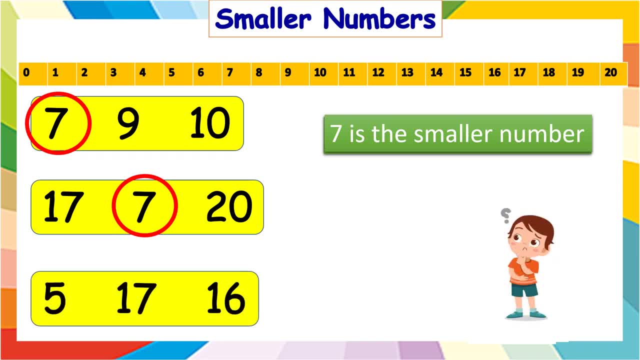 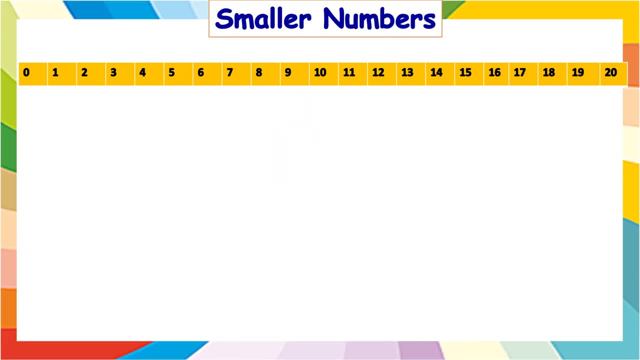 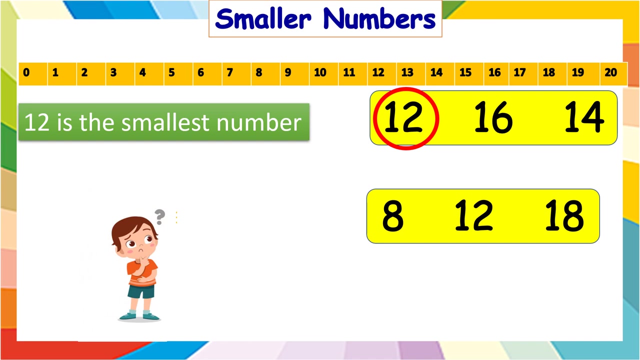 And in five, seven and sixteen. It is five, In twelve, sixteen and fourteen, which is the smallest number, It is twelve. It is twelve right. In eight, twelve and eighteen. It is eight, And in eighteen, seventeen and twelve. 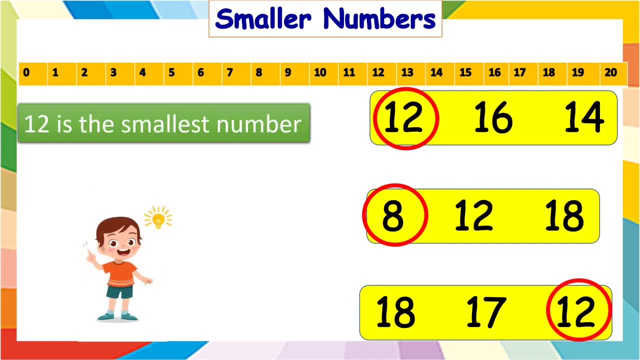 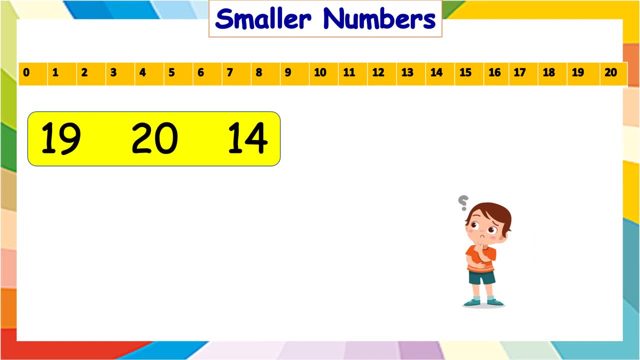 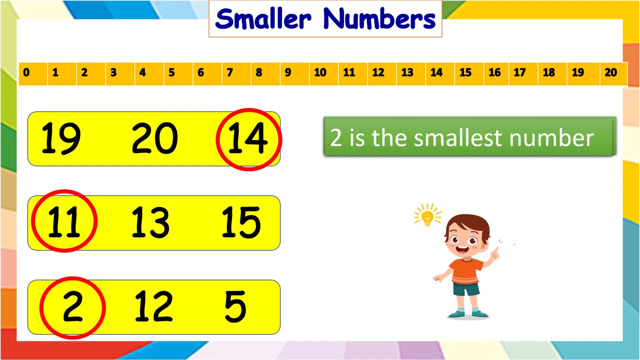 Of course it is twelve, From nineteen, twenty and fourteen, which is the smallest number, It is fourteen. Next, in eleven, thirteen and fifteen, The answer is eleven, And in two, twelve and five It is two. 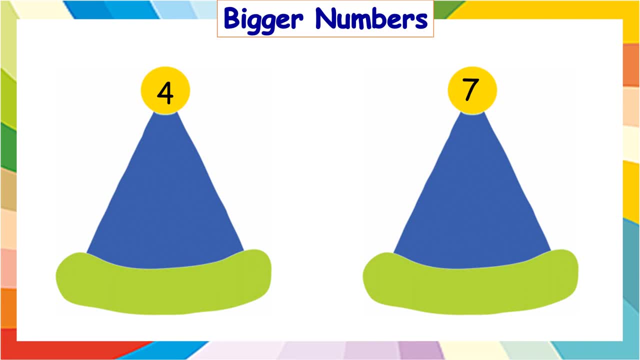 Now it is time to learn bigger numbers. Look at the clown's hat and draw the given number of circles in each hat: One, two, three and four. Now one, two, three, four, five, six and seven. 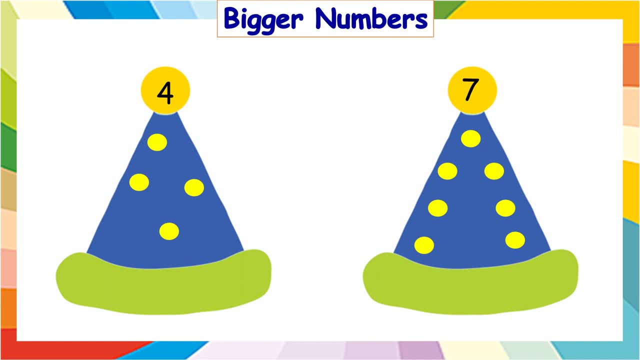 Tell me which is the biggest number, Four or seven? It is seven. Let us draw circles in two more clown's hat. In first hat we need to draw one, two, three, four, five and six circles. 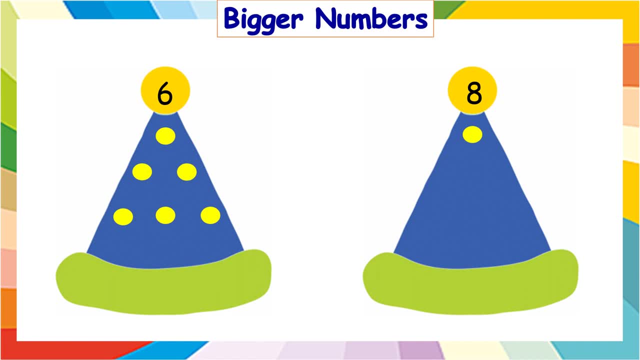 And in second hat there are one, two, three, four, five, six, seven and eight circles. Now tell me which is the bigger number, Six or eight? Eight is the bigger number. Always remember which is the biggest number.